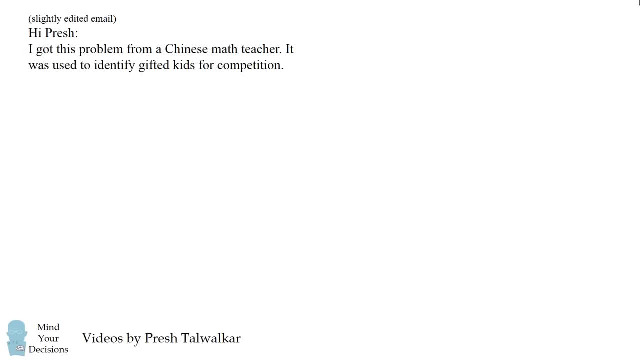 Hey, this is Presh Talwalkar. Here's a slightly edited version of an email I received. Hi, Presh, I got this problem from a Chinese math teacher. It was used to identify gifted kids for competition. ABCD is a parallelogram In the diagram. the areas of yellow regions are 8,, 10,, 72, and 79. 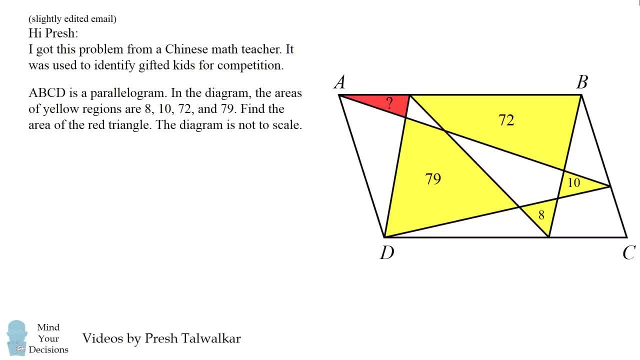 Find the area of the red triangle. The diagram is not to scale. The math prerequisites to solve this problem are basic arithmetic and knowing the area of a parallelogram and the area of a triangle. I was told a few Chinese 5th graders solved it in less than 1 minute. 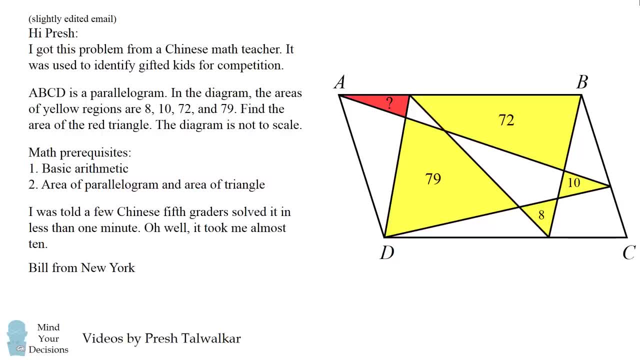 Oh well, it took me almost 10.. Bill from New York, So I gave this problem a try and it was extremely challenging for me and I just couldn't figure it out. So I replied to Bill: I couldn't solve it. Please let me know the solution. 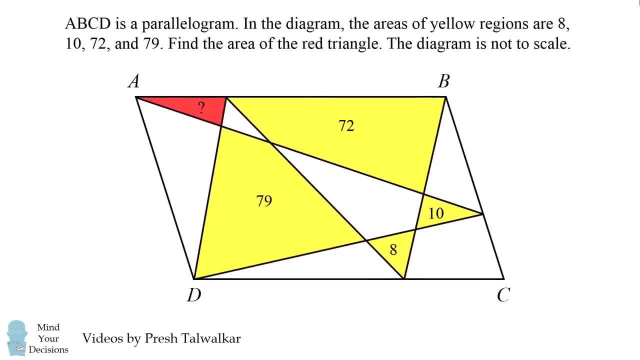 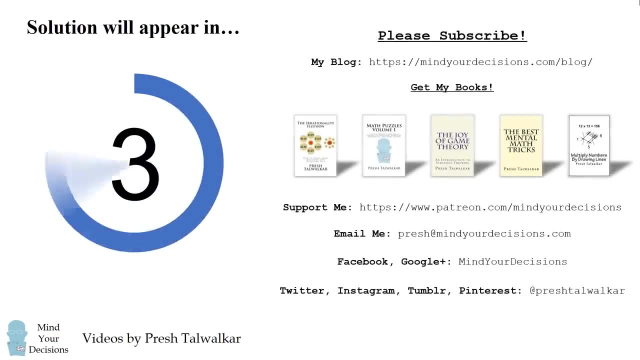 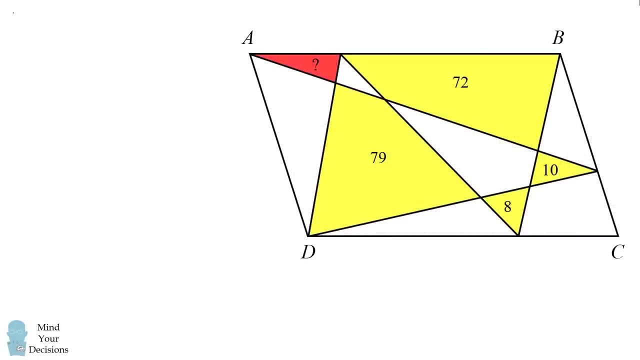 So I'm going to magnify this problem for you and I'm going to ask you: can you figure out this problem? Give this puzzle a try and, when you're ready, keep watching the video for a solution. So here's the magical answer: It turns out to be a simple calculation. 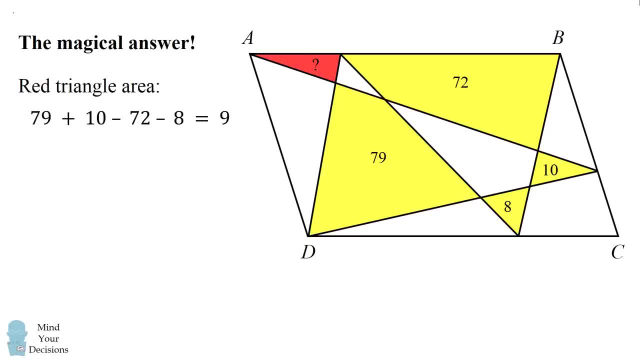 The area of the red triangle is 79 plus 10 minus 72 minus 8,, which equals 9.. Wow, But why is this the answer? It's important to understand the method, to verify the answer and to strengthen problem solving skills. So, even though I didn't find the answer, 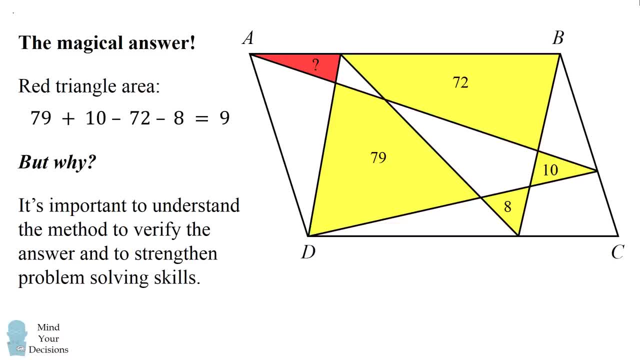 it was very exciting for me to understand how the answer could be solved in such a simple method. Bill explained to me the key is finding a triangle, or set of triangles whose area equals one half the area of the parallelogram. So before I get to the solution, 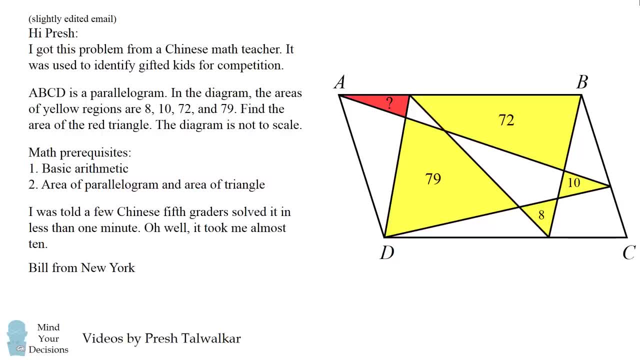 Oh well, it took me almost 10.. Bill from New York, So I gave this problem a try and it was extremely challenging for me and I just couldn't figure it out. So I replied to Bill: I couldn't solve it. Please let me know the solution. 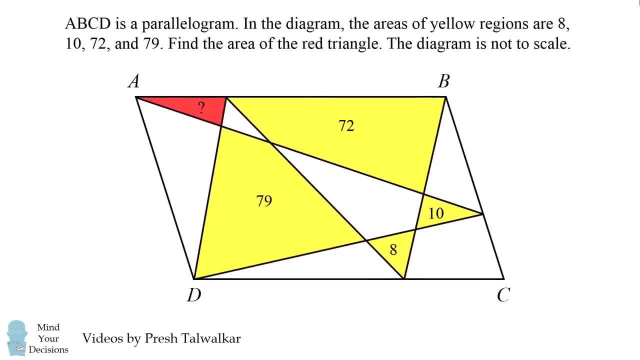 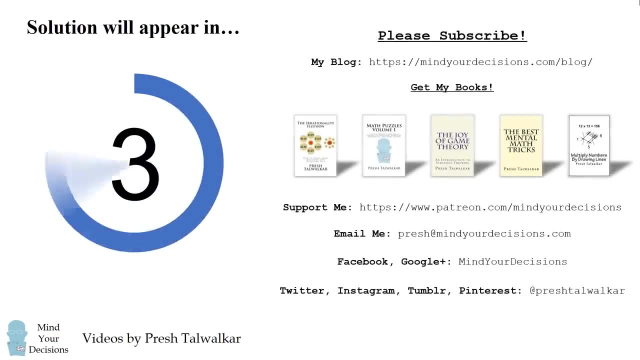 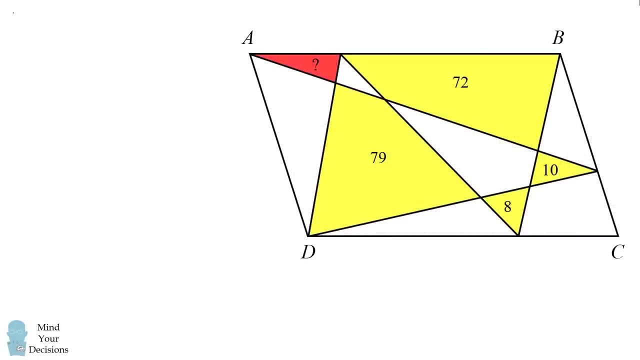 So I'm going to magnify this problem for you and I'm going to ask you: can you figure out this problem? Give this puzzle a try and, when you're ready, keep watching the video for a solution. So here's the magical answer: It turns out to be a simple calculation. 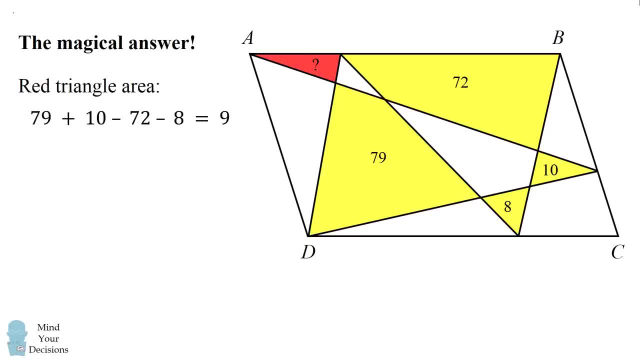 The area of the red triangle is 79 plus 10 minus 72 minus 8,, which equals 9.. Wow, But why is this the answer? It's important to understand the method, to verify the answer and to strengthen problem solving skills. So, even though I didn't find the answer, 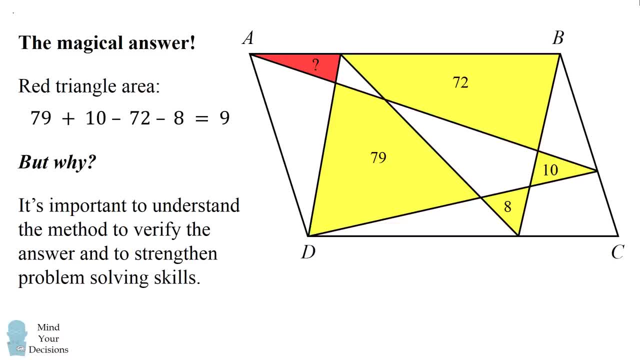 it was very exciting for me to understand how the answer could be solved in such a simple method. Bill explained to me the key is finding a triangle, or set of triangles whose area equals one half the area of the parallelogram. So before I get to the solution, 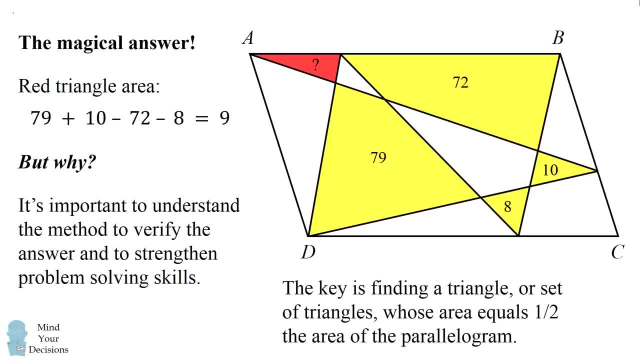 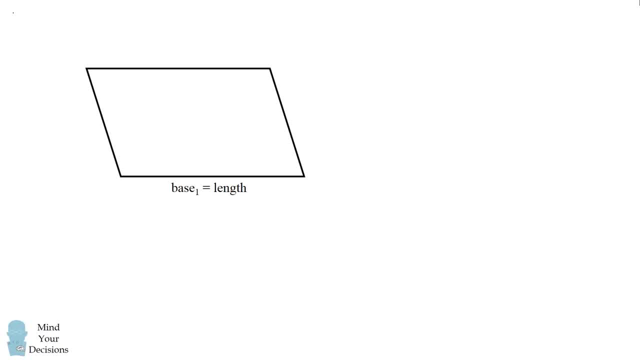 I want to quickly review the areas of a parallelogram and a triangle. So let's take a parallelogram and we'll consider the base of the parallelogram as its length To find the area we draw a vertical altitude as its height. 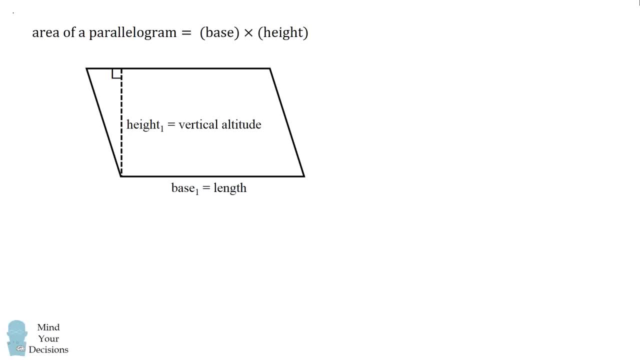 Now, the area of a parallelogram is its base times its height. But we can also calculate it taking the width of the parallelogram as its base. We then draw a horizontal altitude as its height. We then draw a horizontal altitude as its height. 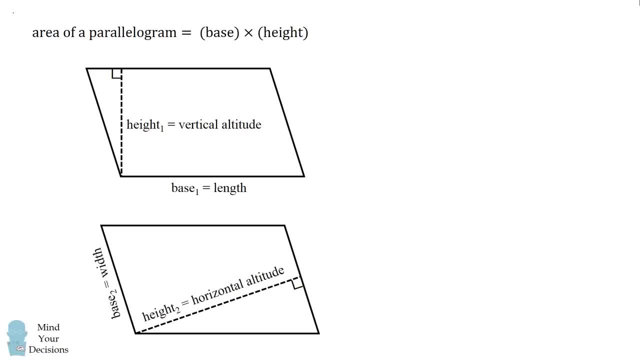 its height, and we then use the same formula of base times height. even though we'll be using different values for its base and its height, this will still give us the area of a parallelogram. now, from this formula, we can deduce the area of a. 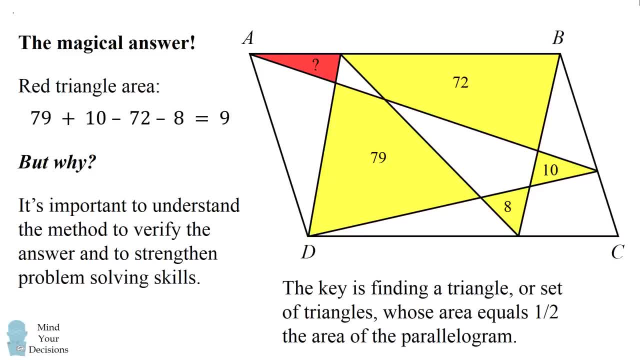 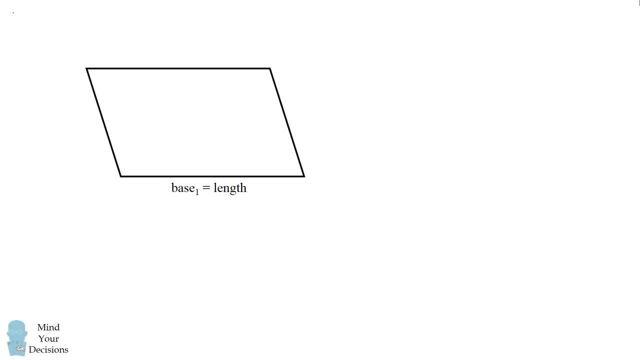 I want to quickly review the areas of a parallelogram and a triangle. Let's take a parallelogram and we'll consider the base of the parallelogram as its length To find the area we draw a vertical altitude as its height. 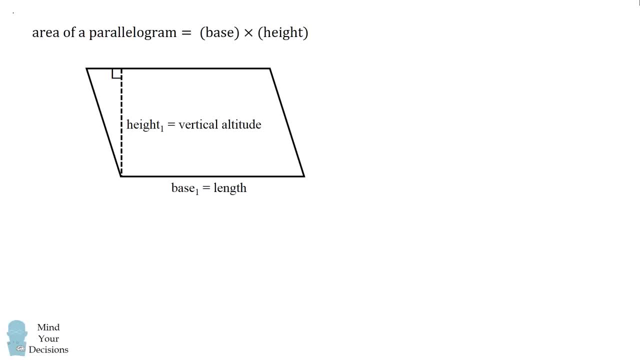 Now, the area of a parallelogram is its base times its height, But we can also calculate it taking the width of the parallelogram as its base. We then draw a horizontal altitude as its height, its height, and we then use the same formula of base times height, even though we'll be using 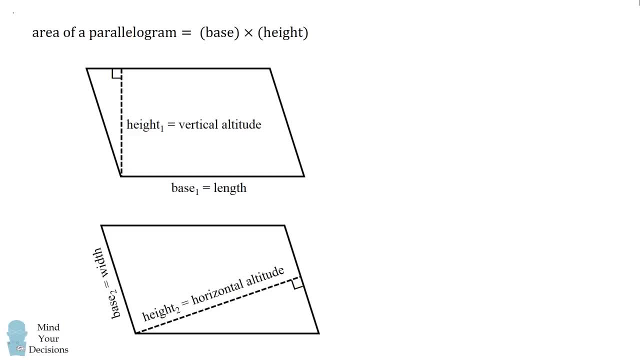 different values for its base and its height. this will still give us the area of a parallelogram. now from this formula we can deduce the area of a triangle. let's draw the diagonal of this parallelogram and notice we split it into two equal triangles, so the triangle has half the 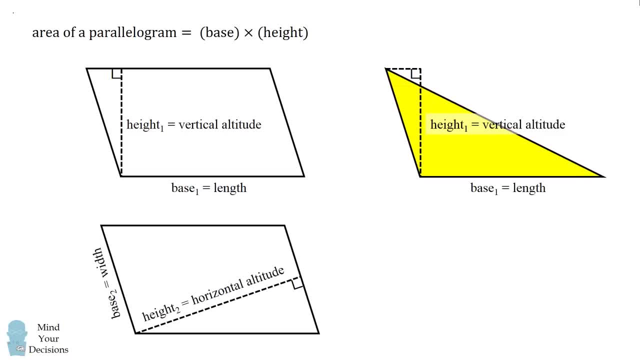 area of the parallelogram. therefore, the triangle has an area that's equal to base times the height divided by two. we can also use the formula: if we take the base of the triangle as the width of the parallelogram, we then will want to use the horizontal altitude as the height, so we can use 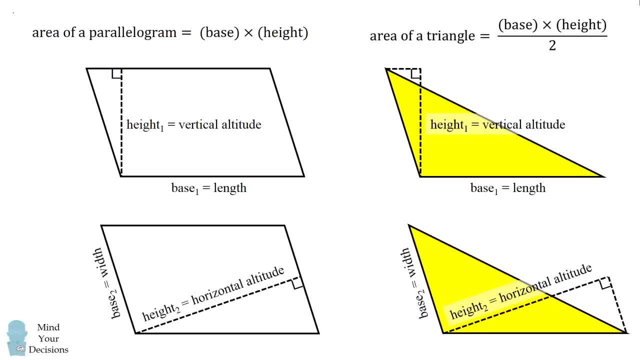 the formula base times height divided by two, but we can look at different sides as the base. furthermore, this formula will be true for a triangle that's not even the diagonal of the parallelogram. as long as it has the same base and the same height, we will still get half the area of the 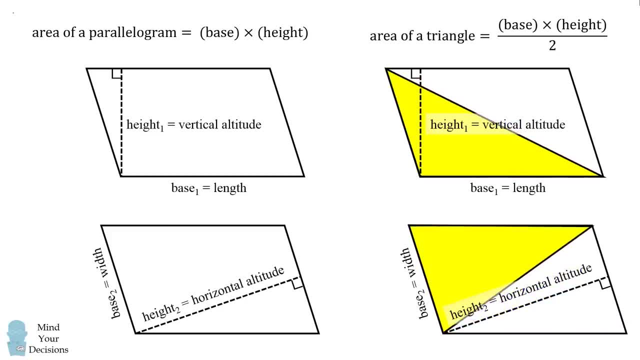 parallelogram, so keep this in mind. it'll be a very useful principle for solving this problem. one more thing that'll be useful is that it doesn't just have to be one triangle. imagine we have a set of two triangles that span the length of this parallelogram, and both 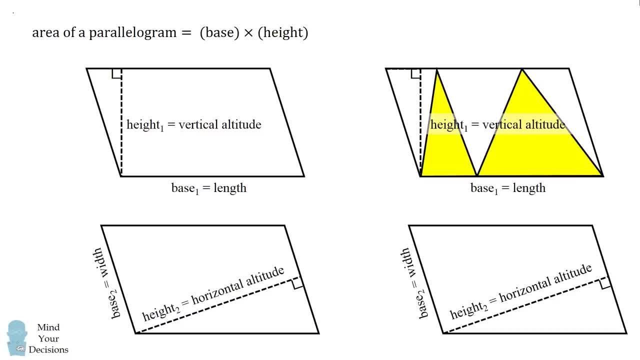 of them have the same height as the base of the parallelogram, so we can get half the area of the parallelogram the same height as the parallelogram. so the sum of these two triangles areas will again be equal to the base times the height divided by two, and this will also be equal to half the area of the. 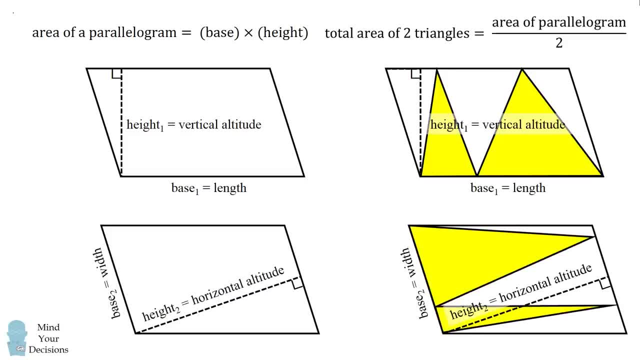 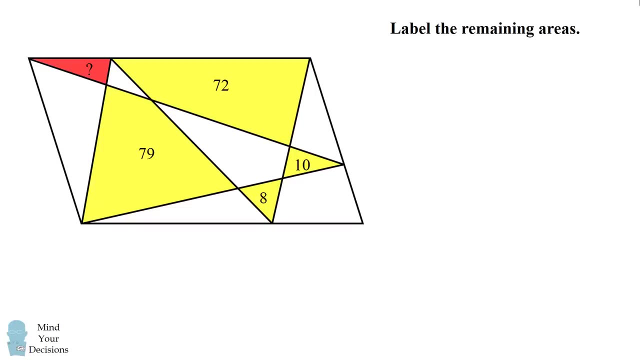 parallelogram. this will also be true if we take two triangles that span the width of the parallelogram. so now let's use these principles to solve the problem. we go to our diagram and the first thing we'll do is we'll label. the remaining areas, we'll write. 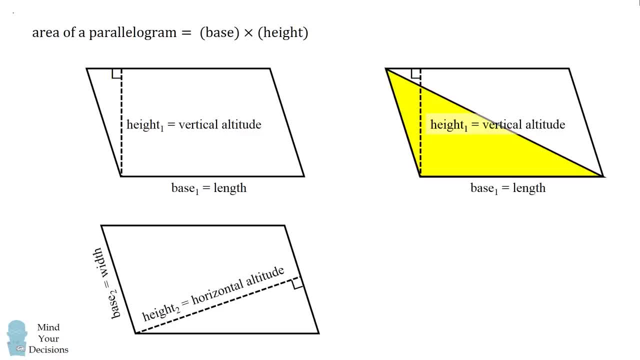 triangle. let's draw the diagonal of this parallelogram and notice we split it into two equal triangles, so the triangle has half the area of the parallelogram. therefore, the triangle has an area that's equal to base times the height divided by 2. we can also use the formula, if we take the base of the triangle as: 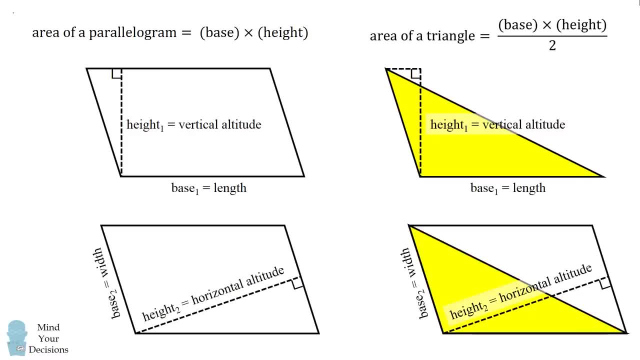 the width of the parallelogram. we then will want to use the horizontal altitude as the height, so we can use the formula base times height divided by 2, but we can look at different sides as the base. furthermore, this formula will be true for a triangle. that's not a triangle. but it's a triangle, that's not a triangle. 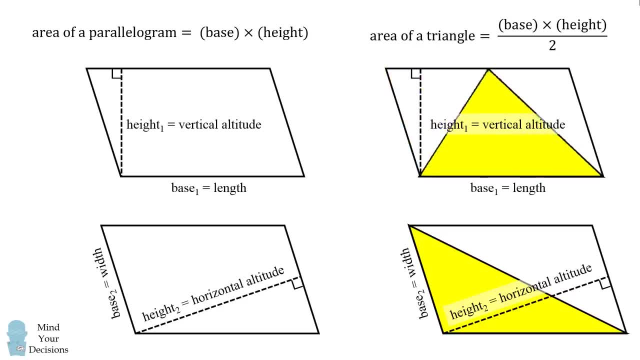 it's not even the diagonal of the parallelogram. as long as it has the same base and the same height, we will still get half the area of the parallelogram, so keep this in mind. it'll be a very useful principle for solving this problem. one more thing that will be useful is that it doesn't just have to. 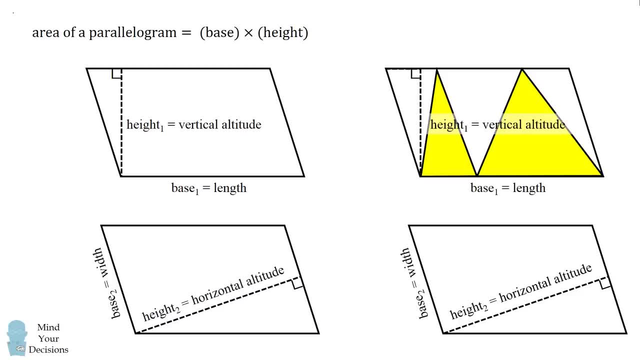 be one triangle. imagine we have a set of two triangles that span the length of this parallelogram, and both of them have the same height as the parallelogram, and then we have a set of two triangles that span the length of this parallelogram. 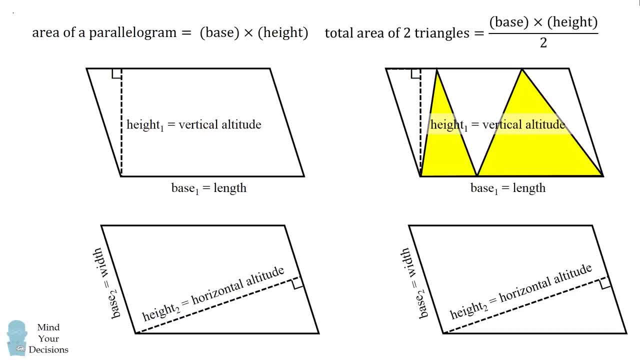 so the sum of these two triangles areas will again be equal to the base times the height divided by 2, and this will also be equal to half the area of the parallelogram. this will also be true if we take two triangles that span the width of the parallelogram. so now let's use these principles to solve the. 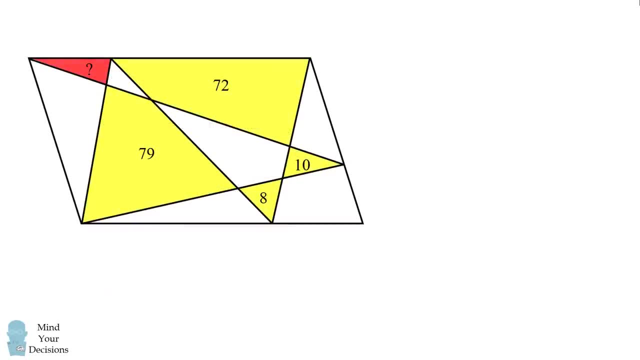 problem. we go to our diagram and the first thing we'll do is we'll label the remaining areas, we'll write ABC, D, D, E and F, and we'll change the question mark, the red triangle, into the variable x. We want to solve for x. So how do we do that? Well, let's look for some triangles whose area 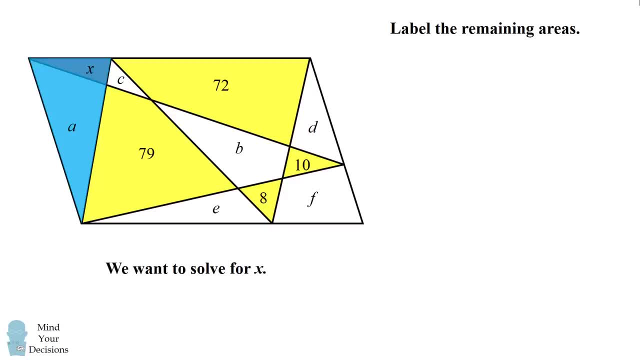 will be half the parallelogram. One set of triangles will be these two blue triangles. They span the length of the parallelogram and they have the same height as the vertical altitude of the parallelogram. So if we focus on just these two triangles, we can see that their area 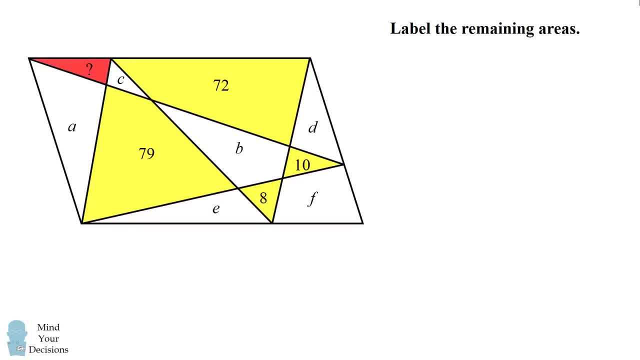 a, b, c, d, e and f, and we'll change the question mark, the red triangle, into the variable x we want to solve for x. so how do we do that? well, let's look for some triangles whose area will be half the parallelogram. one set of triangles will be these two blue triangles. 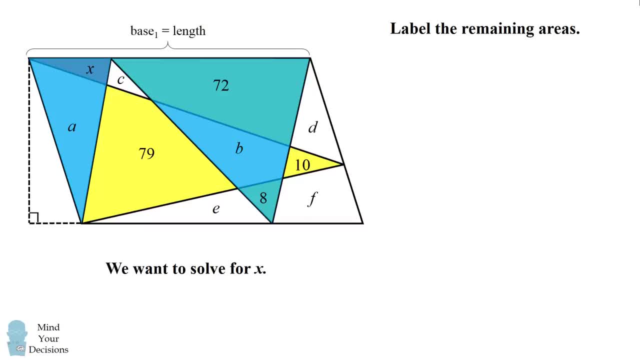 they span the length of the parallelogram and they have the same height as the vertical altitude of the parallelogram. so if we focus on just these two triangles, we can see that their area will be half the area of the parallelogram. and we can also calculate their area by adding up these letters. we have x plus a plus 72. 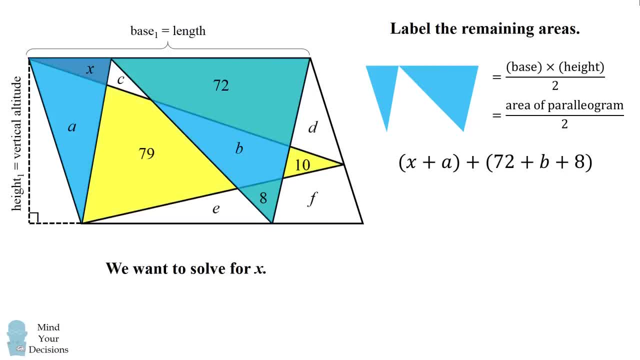 plus b plus 8.. now let's look for another triangle whose area is half the area of the parallelogram. consider this orange triangle here. this orange triangle spans the width of the parallelogram and its height is equal to the horizontal altitude, so its area will also be half the area of the parallelogram. we can write out its. 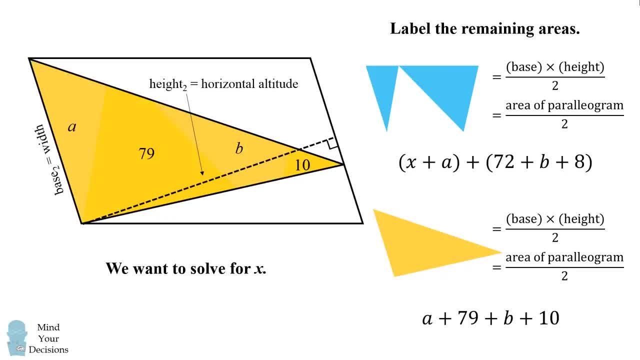 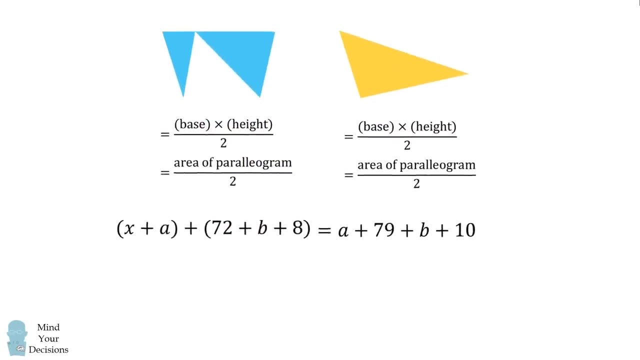 area as a plus 79 plus b plus 10.. now both of these sets of shapes have an area that's equal to half the area of the parallelogram. so we can say that the area of the parallelogram is equal to the parallelogram. so we can set these areas equal to each other. so we equate these two formulas for 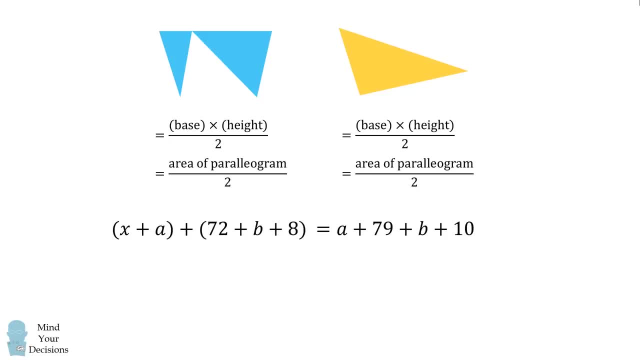 the half the area of the parallelogram. and now we can solve for x. notice that on both sides we have an a, so these will cancel. on both sides we have a b, so these will cancel. so we end up with the equation: x plus 72 plus 8 is equal to 79 plus 10.. 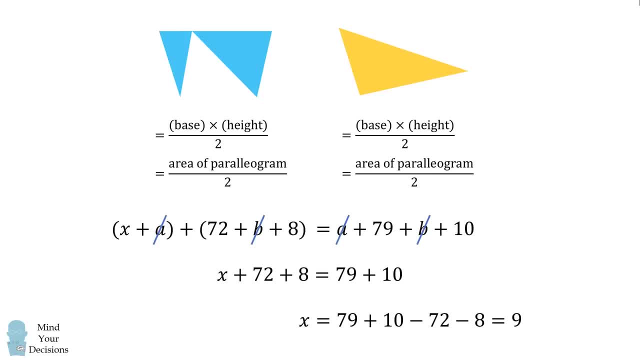 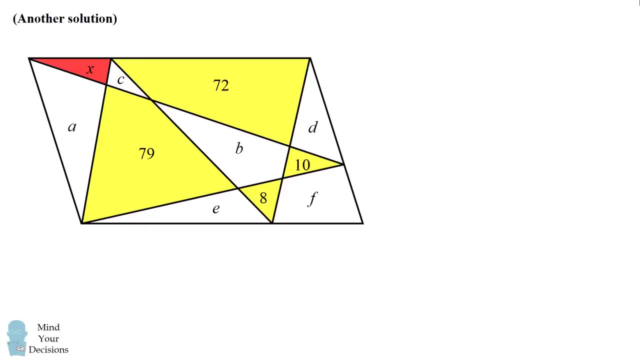 we then solve for x to get 79 plus 10 minus 72 minus 8, which equals 9, and that's how we get the magical answer. but there's also another way if you pick some other triangles. so i just want to illustrate that for you, because bill also sent that to me. so imagine you take these two triangles. 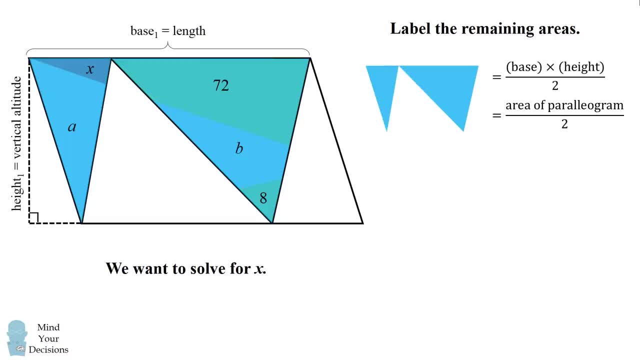 will be half the area of the parallelogram, and we can also calculate their area by adding up these letters. We have x plus a plus 72 plus b plus 8.. Now let's look for another triangle whose area is half the area of the parallelogram. 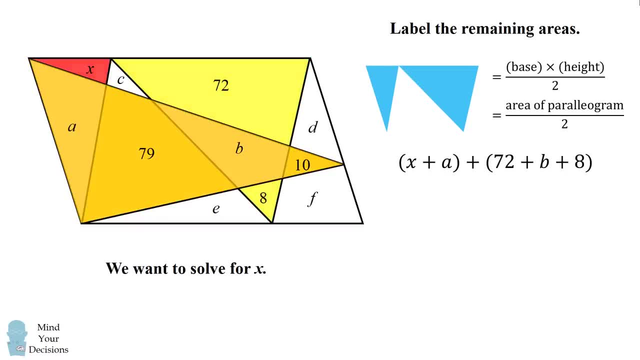 Consider this orange triangle here. This orange triangle spans the width of the parallelogram and its height is equal to the horizontal altitude, So its area will also be half the area of the parallelogram. We can write out its area as a plus 79 plus b plus 10.. Now both of these sets of shapes. 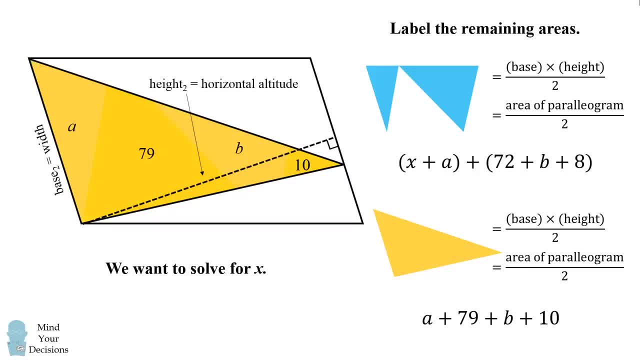 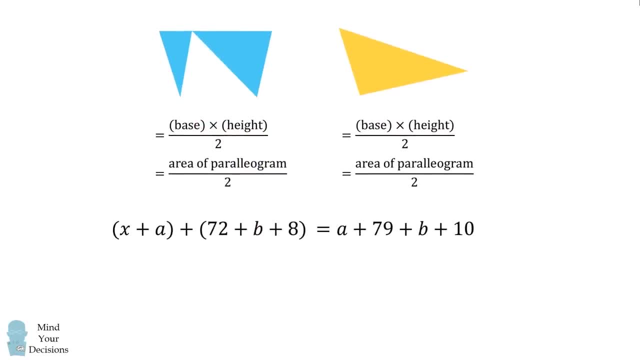 have an area that's equal to half the area of the parallelogram. So we can set these areas equal to each other. So we equate these two formulas for the half the area of the parallelogram. and now we could solve for x. Notice that on both sides we have an a. 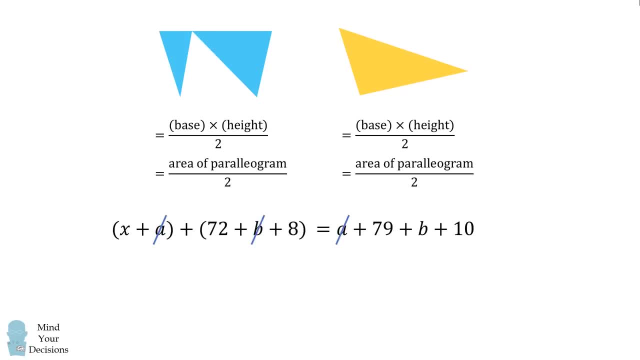 so these will cancel. On both sides we have a, b, so these will cancel. So we end up with the equation: x plus 72 plus 8 is equal to 79 plus 10.. We then solve for x to get 79 plus 10 minus 72 minus 8, which equals 9.. 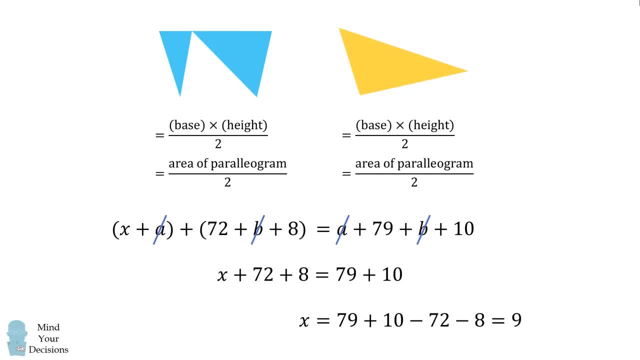 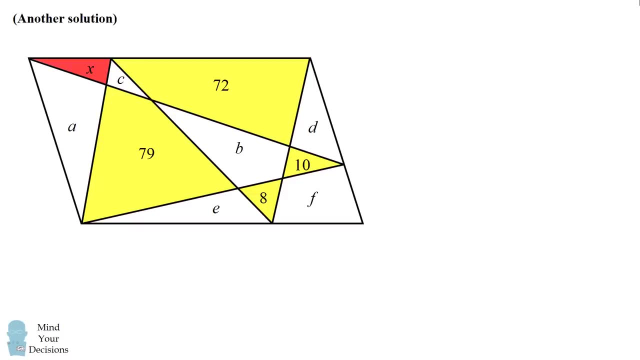 And that's how we get the magical answer. But there's also another way if you pick some other triangles. So I just want to illustrate that for you, because Bill also sent that to me. So imagine you take these two triangles. These two triangles span the length of the parallelogram. 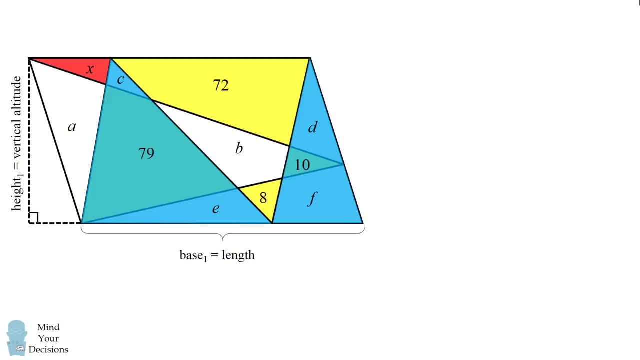 and they have a height equal to the vertical altitude of the parallelogram. Therefore, their area will be equal to half the area of the parallelogram. The areas of these two triangles in total will be c plus 79 plus e plus d plus 10 plus f. 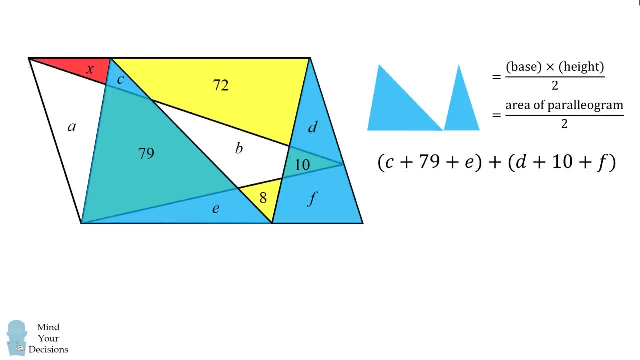 Now we'll do the same thing. We'll consider a different triangle, or a different set of triangles along the width of the parallelogram. So these orange triangles will have a base that's equal to the width of the parallelogram and they span the horizontal altitude of the parallelogram.